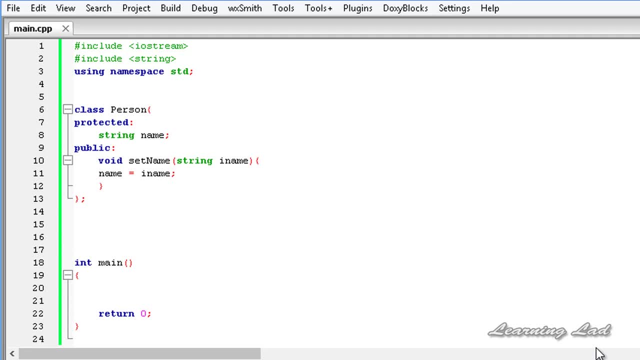 Hi, this is Anil and welcome to the video tutorial for the learning light on C++ programming. So in this tutorial we're going to learn about the protected inheritance. So in the previous tutorial we have learned about the public inheritance. You know, when we use the public. 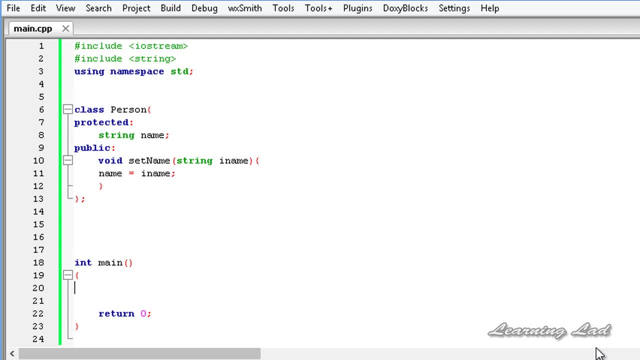 inheritance, all the public and protected members of the base class are going to act as the public and the protected members of the derived class respectively. So here, when we use the protected inheritance, you know the public and also the protected members of the base class are going to. 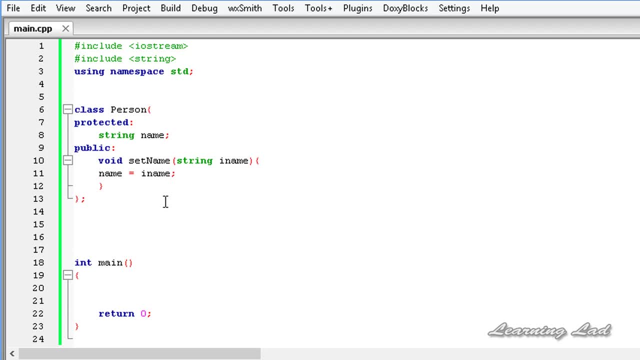 act as the protected members of the derived class. So if it is confusing, don't worry, you know, let's see with the example. So here, for the demonstration purpose, I have a class called person And as a protected member I have name and as a public method I have set name, you know. 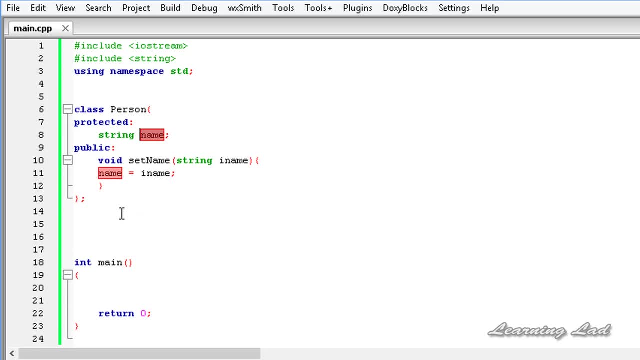 which is going to set the value to this protected member name. So here, to demonstrate the protected inheritance, I'm going to create a class called student. You know, here we're going to be having the protected inheritance. That's why we need to use the keyword protected, while 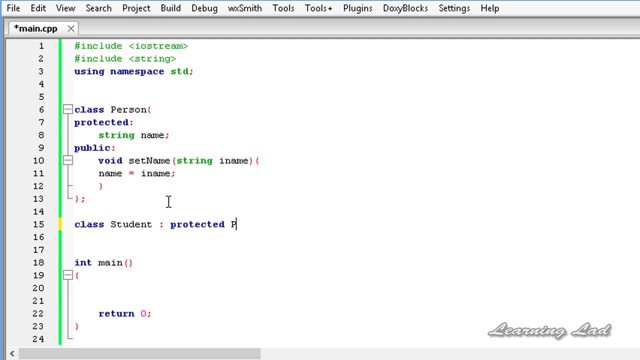 inheriting from the base class and then the base class name, which is person, And here in this class, student. let's have a public method And let's call it as display. And you know, this display method is going to display the value of this base class member name. So 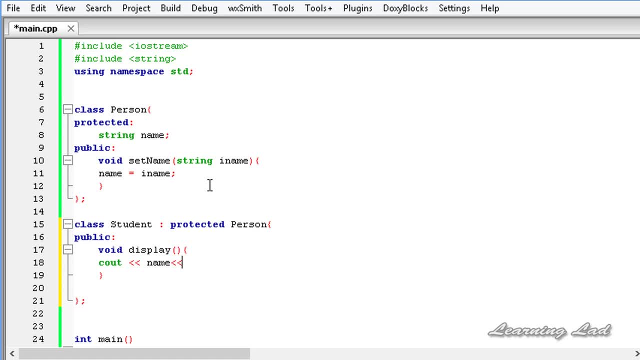 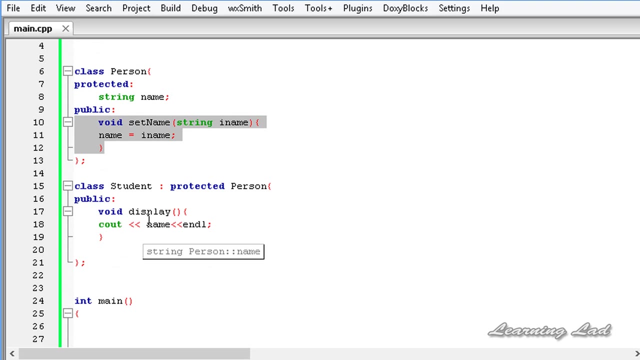 it's going to be cout And let's call it as name and end this line All right. Now, when we use this protected inheritance, you know the public and also the protected members of the base class are going to act as the protected members of this derived class, which is nothing, but you know. 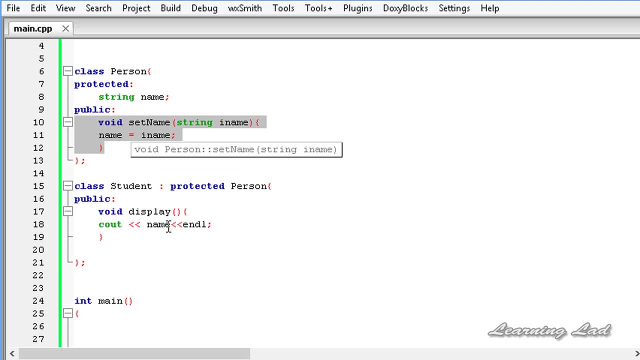 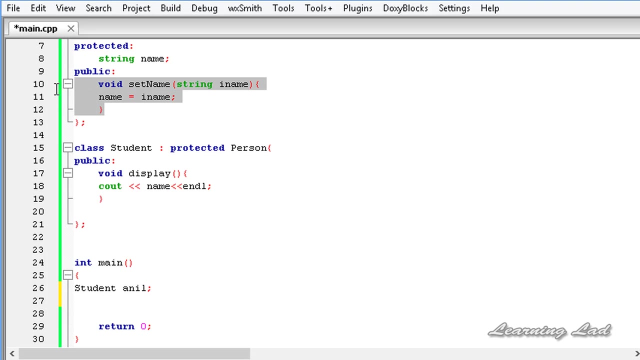 this public, members of the base class are going to become the protected members in the derived class. So, just to demonstrate that, what I'm going to do is I'm going to create an object of this class student. So it's going to be student, And let's call it as Anil. Now, this public 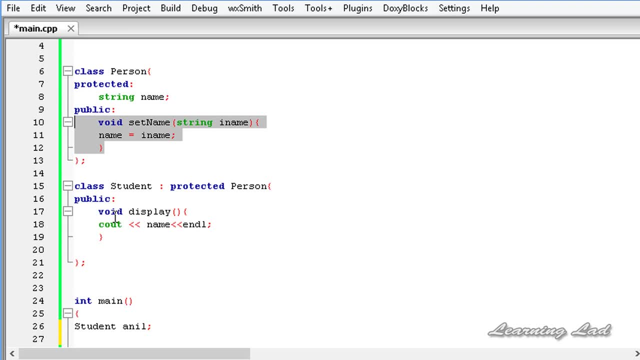 method of this base class person is going to become the protected method of this derived class student, And that's why I can't access the set name method here. If I try to do that, I'll get the error. Just to demonstrate that what I'm going to do is I'm going to write.